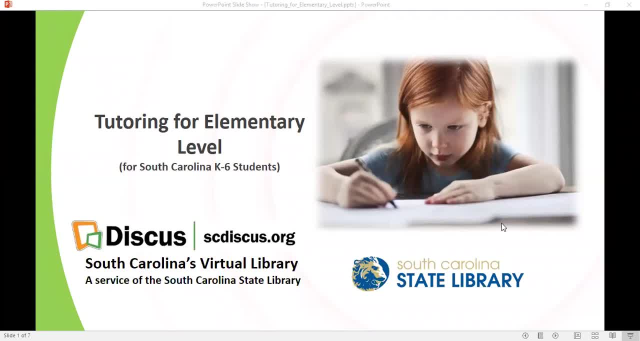 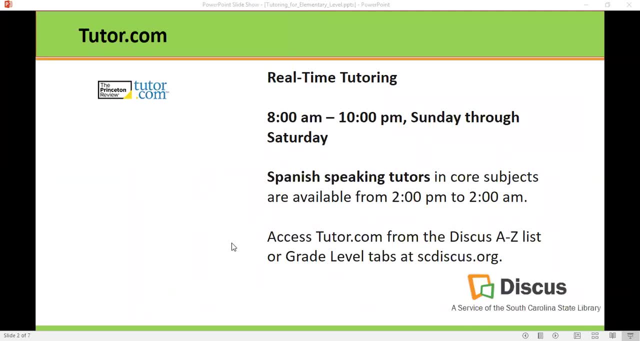 share the recording out just to get the word out to your schools. So tutorcom is actually available on the South Carolina State Library. It's available on the South Carolina State Library to K through 12 students in South Carolina and these on your screen are the tutoring times from: 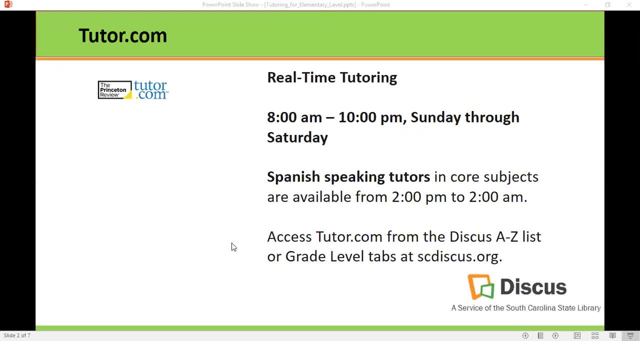 8 am to 10 pm Sunday through Saturday. If a student tries to access after 10 pm, there is a notification on the screen that will tell them that the tutors will be available again at 8 am. 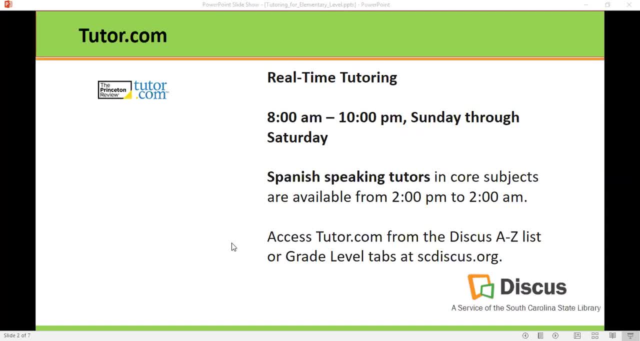 There are also Spanish-speaking tutors that are available from 2 pm to 2 am, And again with our elementary students especially, that would be up to the parent or guardian's decision as to how late they would actually want want the student to use this, But this, those are. 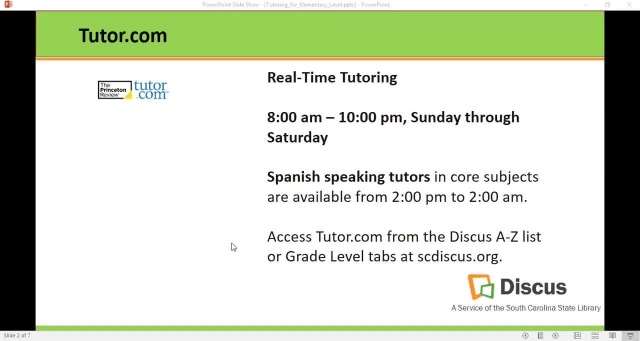 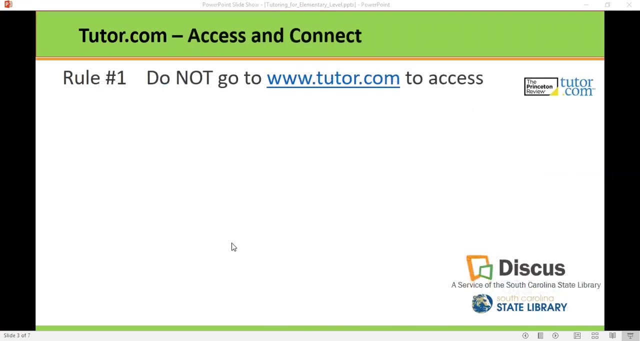 those, those two tutors that speak Spanish for the students whose first language is Spanish. So if they would do better getting something explained in that language. You can access tutorcom from the Discus. You can access it from the C, C, C listed or the grade level tabs at our site. It's very important that you do not go to wwwtutorcom to access. 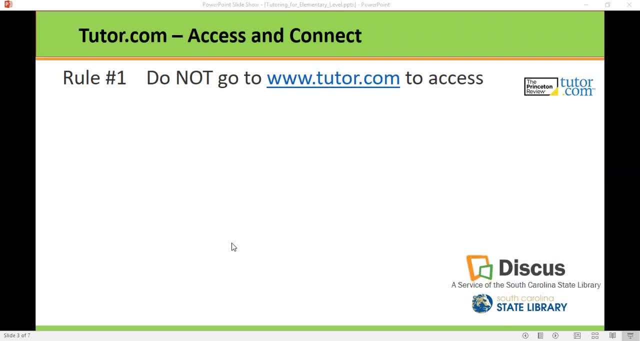 That's one of the things that we've discovered. It has kind of been a misunderstanding, a bit of confusion, Because the name of the product is tutorcom and we all, by nature, are going to go out to, you know, to the website of whatevercom we hear. 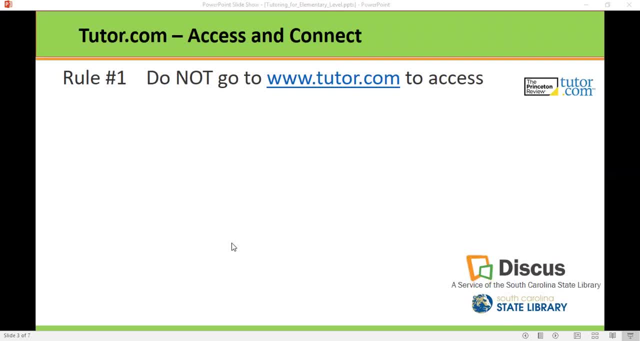 if you're ever working with a patron or working with a student and you know the first thing they say is: I cannot connect to a tutor, you're going to know that this- this would be the first thing for you to check- is just to make sure that they are going out to our through the Discus. 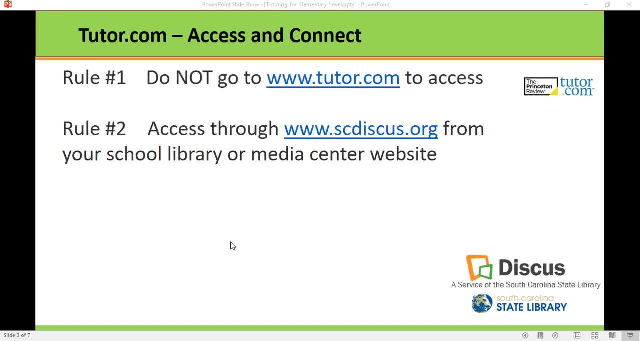 website. So that would be rule number two: access through scdiscusorg from your school library or media center website. That said, for those of you who are at the schools, you can also access tutorcom from their public county library, but there's going to be a different access point. 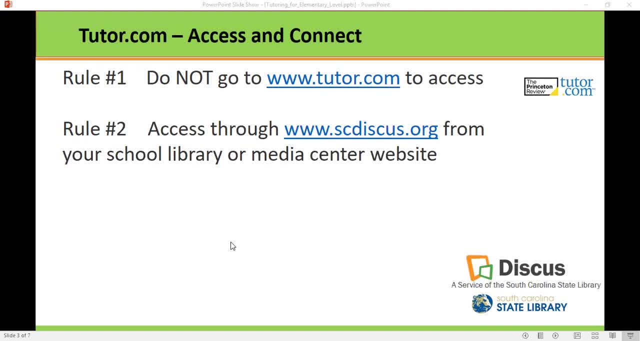 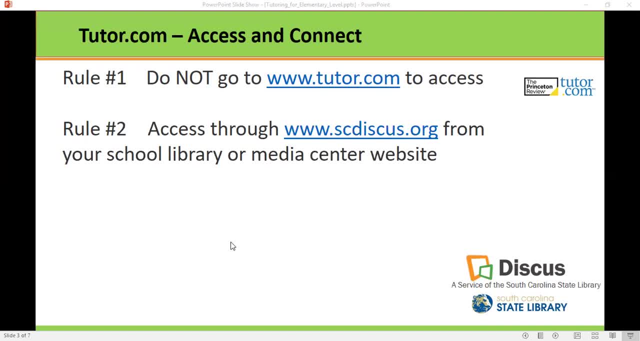 like to just reinforce and get the students and parents in the habit of going through Discus from the contact point at their school so that they get the correct screen. So these are those contact points. They can get it from the A to Z list listed alphabetically from either of the 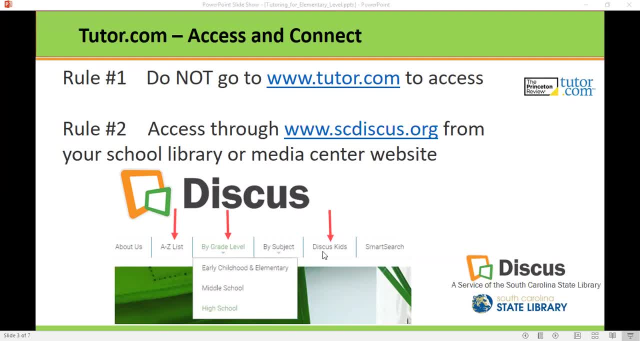 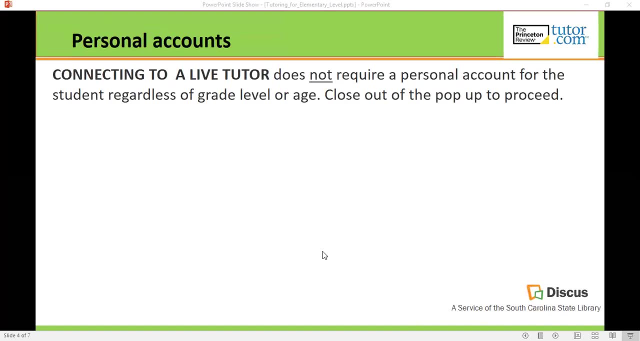 three grade levels or from the Discus kids listing of the of the tutorcom. So that's the first important point that we'll make there. Personal accounts: This is another piece that sometimes is confusing to the students and the parents When you first go and connect, to connect to a tutor which we will go live and do in a 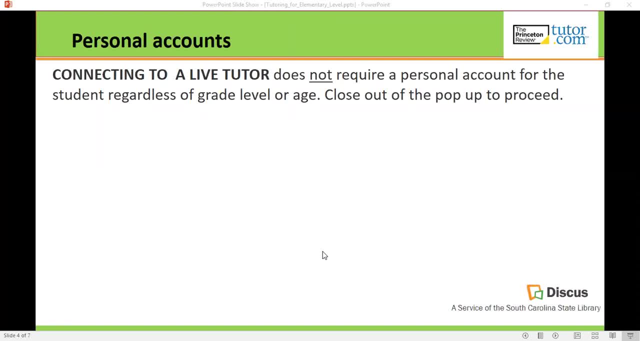 moment we won't actually connect to a tutor, but I'll show you how to do it. When you connect to a live tutor, it does not require a personal account for the student, regardless of their grade level. So you would just want to close out of the pop-up. So whenever they click on connect to a tutor and 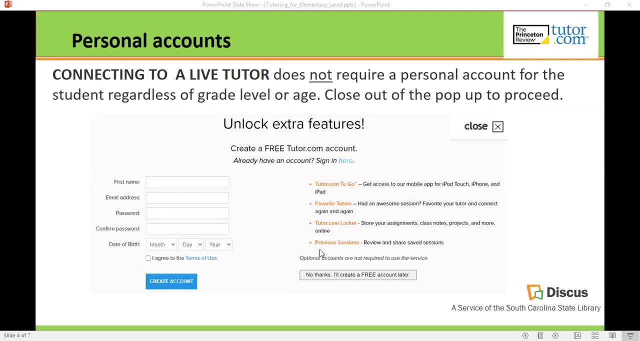 they get this pop-up. you're just going to want to direct those students to close out of that little pop-up. It is not a requirement for them to have that account. In fact, for your elementary level students who are kindergarten through sixth grade and who are 13 years or under, they do not create. 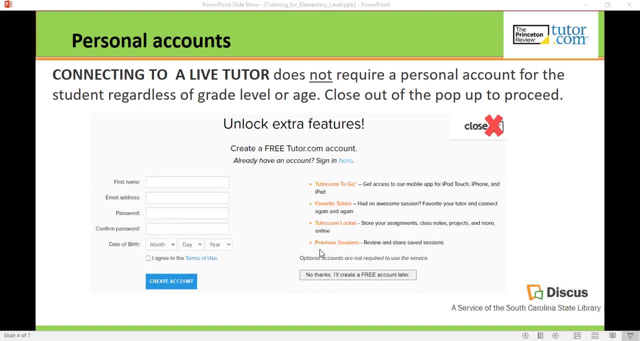 an account. There are different COPA compliant reasons for that, because they're they're actually using emails for those accounts. So that's one. two of the pieces to clarify is just: the access is through the Discus site and you would just close that And we'll. we'll see that again live in a moment. Here is a a couple of. 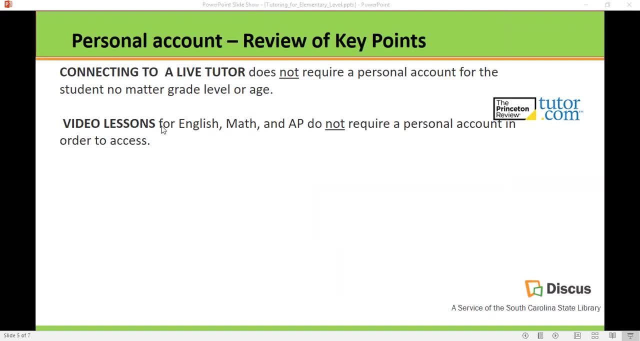 review for these key points. The video lessons for English, math and AP do not require a personal account. If you have a personal account, you're going to have to go to the Discus site and you're going to have to go to the Discus site. 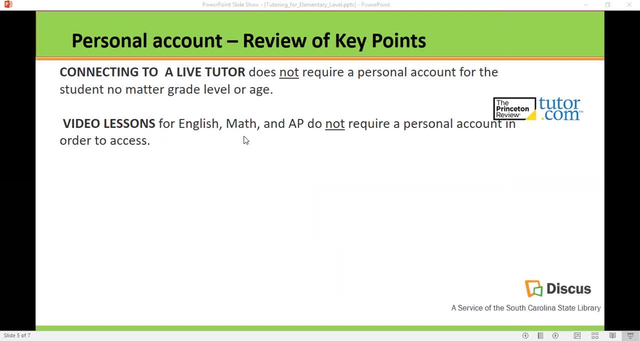 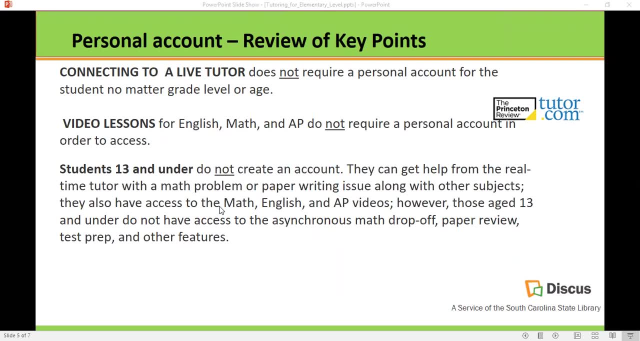 The video lessons for English, math and AP do not require a personal account either, And we'll we'll actually look at that live in a moment. This is a statement that I do like to put up here for everyone to know, that students 13 and under do not. 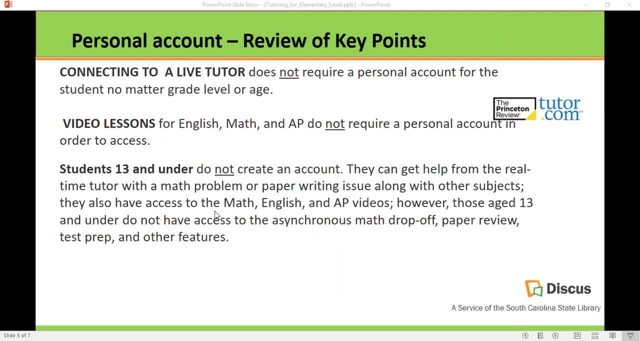 create an account, They can get help from the real-time tutor with a math problem or paper writing issue, along with many other subjects. They also have access to the math, English and AP videos, which they're probably not going to want. the advanced placement. 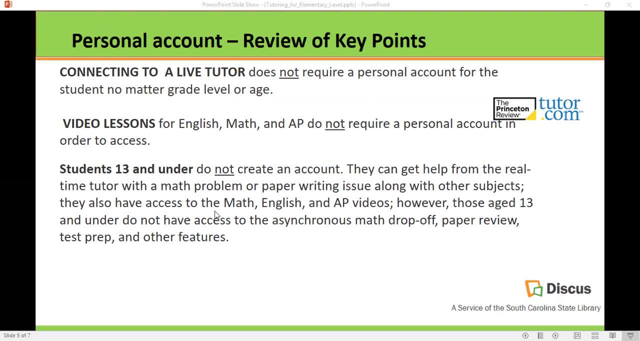 videos yet, But those are not. also do not require an account. However, those age 13 and under do not have access to the asynchronous math drop off paper review, test prep and other features, So I'm going to show you. it always helps to see the visual of that, but this is just some text and key points that you can use. 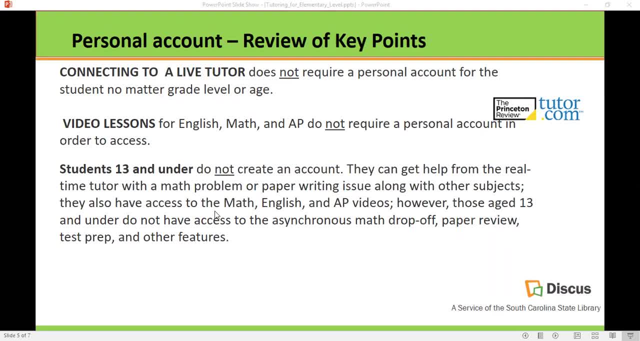 also, I will also throw in there for you all who are media specialists, teachers at schools, If any of you would like the a copy of these slides to be able to tailor for your own purposes in any of the trainings you do for your school. you're you're welcome to email me for those, those as 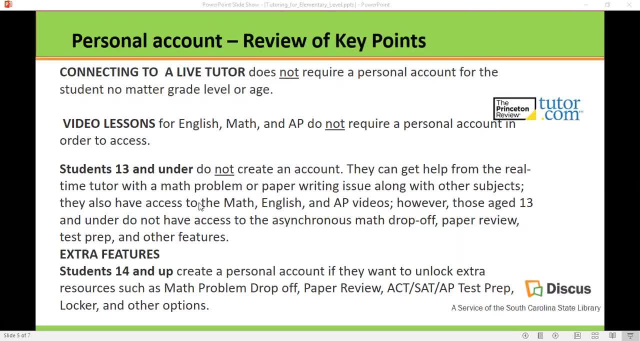 well, I did want to add that students 14 and up can create a personal account if they want to. Again, they can connect to the tutor without having to do that, But if they want to drop a math problem off when the tutors are, 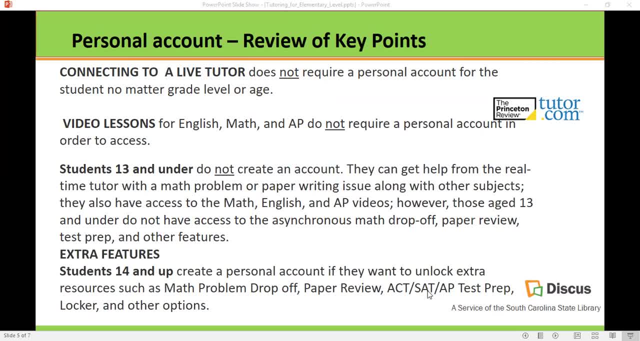 not available or a paper review, etc. Some of your parents will actually have more more children in at the home or in their family than just their elementary student. they may have a 15 year old. So if you do get questions about that, I wanted to clarify that those students do have a couple of more options in tutorcom. 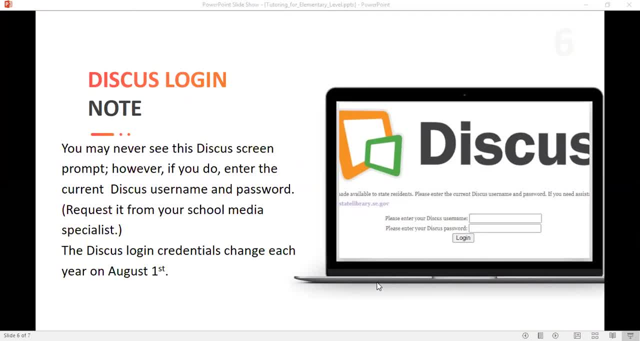 I also want to do a little clarification. clarification on the third piece, the screen that I just showed you prior to this that had the account where it had the unlocked the extra features account. We do have some parents and students who think that means they need to enter the discus username and 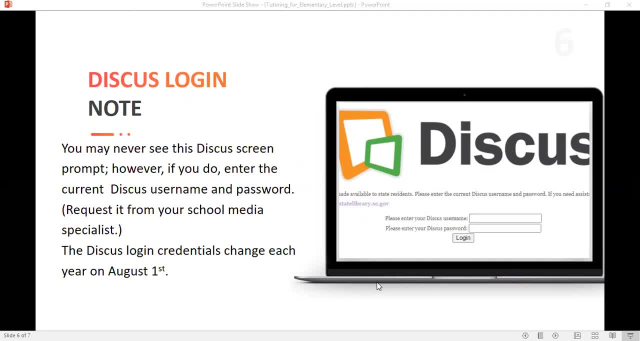 password And that causes a bit of confusion. So if you're ever helping a parent or a student, you want to make sure that they know they do not enter the discus account. the only they would need to enter that Discus account is if they see this screen. that's prompting them. 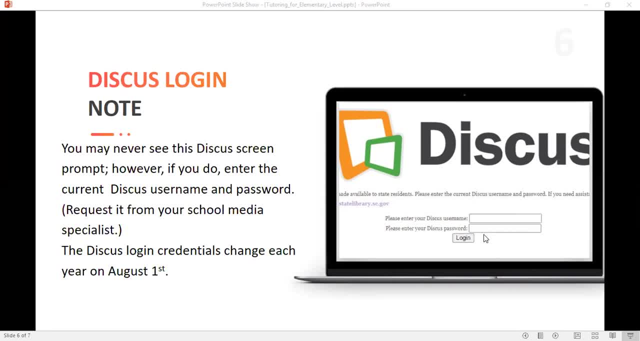 And, as you all know, as media specialists, sometimes that happens if they're on a remote device or not using one of the computers at the school, those kinds of issues. But just to make that distinction that they should not need the Discus username and password to connect to the 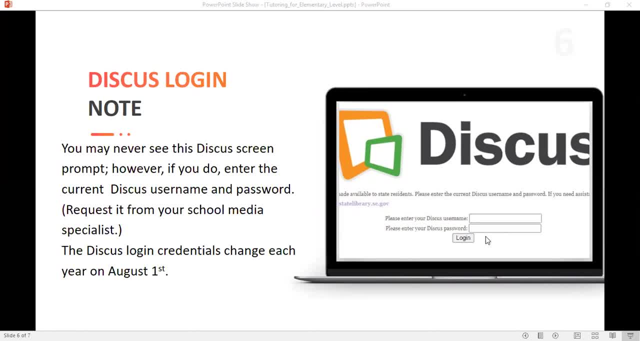 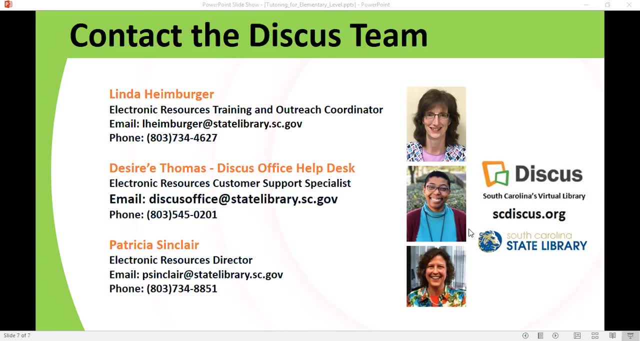 tutor, but if they ever get prompted by this screen. Okay, so that was some of the do's and don'ts. Now we're going to go ahead and go live. I'm going to stop the share on this screen and we are going to go ahead and go live there to the interface. So let me just do a new share here. 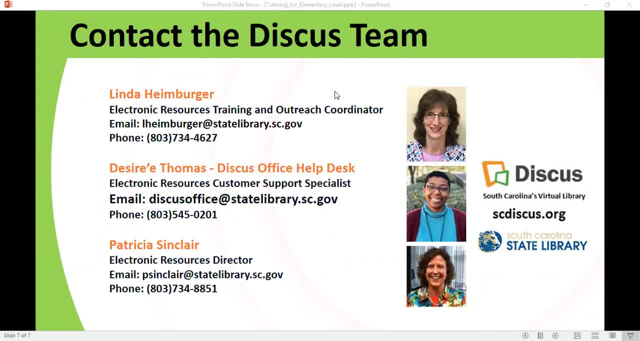 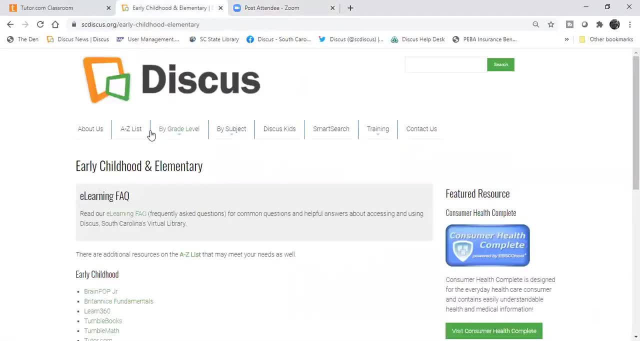 and I'll pull this up for us. So again, you can access through the A to Z list. You can access through grade levels or through the Discus Kids listing of databases. I'm just going to quickly jump into A to Z list: click on the. 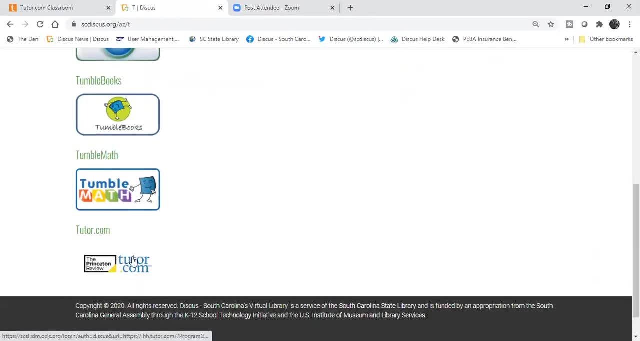 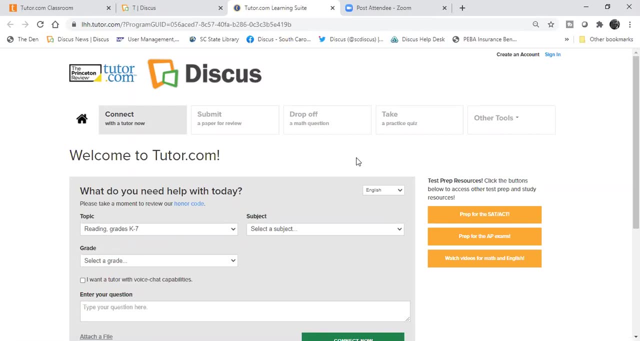 letter T and go down to tutorcom. So the very first thing that you should see whenever you're- you all know this- is that you're going to want to make sure that you have access to the Discus logo. You go to tutorcom, a student goes to tutorcom- is that Discus logo? That way, you 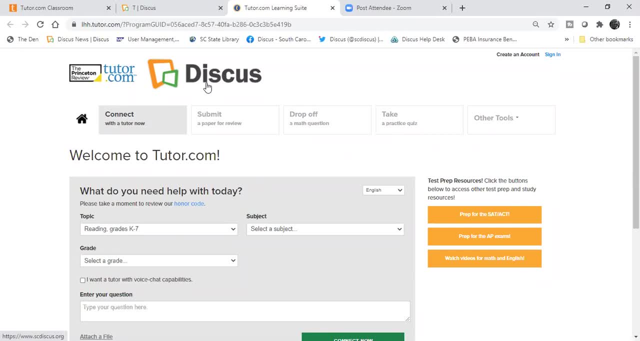 know they have accessed it correctly. So that's one of the first things to ask as a troubleshooting piece. If a parent calls and says that they you know that they can't connect or they're having, you know, an issue with that, that's the first thing you want to ask them. Do you see the Discus? 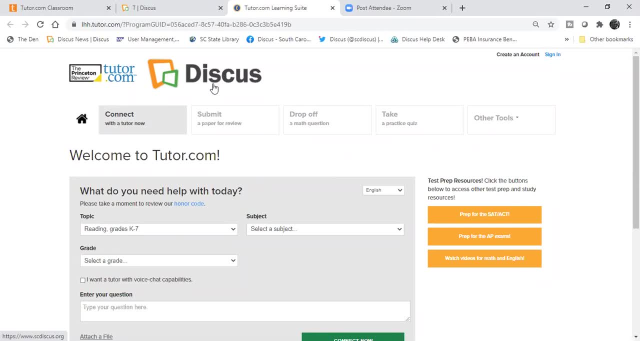 logo at the top If they've gone out to tutorcom instead of going through the Discus site. that way you know they have access to it correctly. So that's one of the first things to ask. as a logo will not be there, Notice across the top here. connect with the tutor now is bolded in. 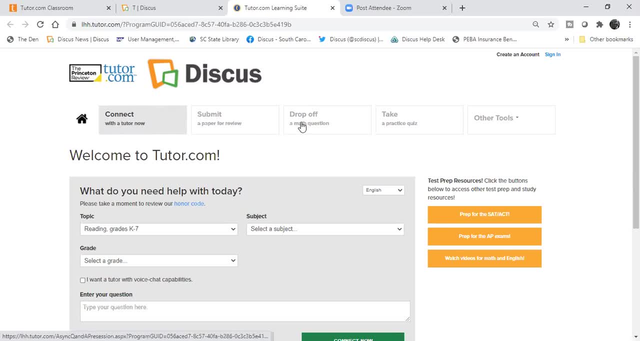 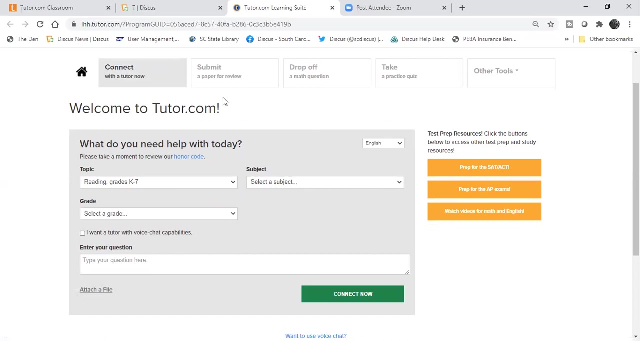 dark print. The other features- to submit a paper, drop off etc. are grayed out. So, again, those are going to be the special features that are optional for the 14-year-olds and up. The videos that are also available to the students without needing an account are the videos for Math. 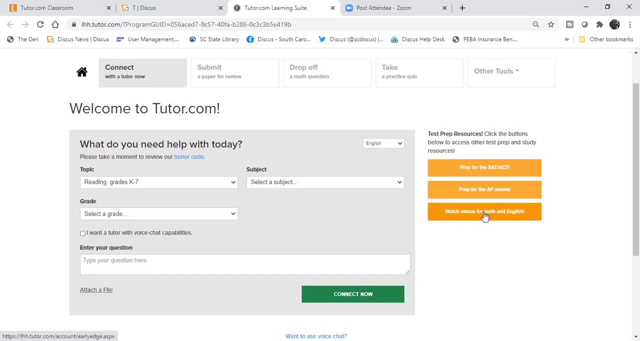 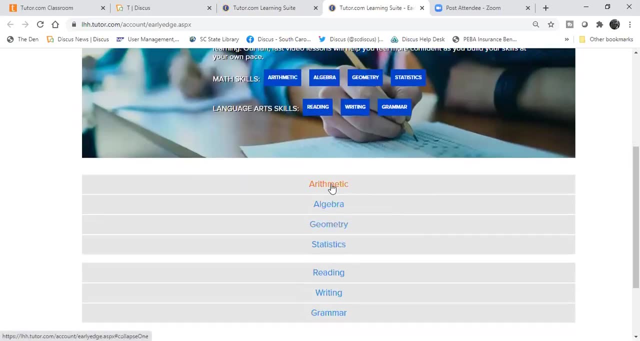 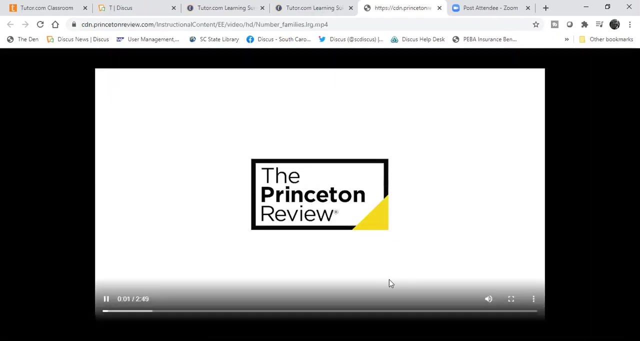 and English that you see on the third orange box on your right. So those videos are broken out here and they're easily accessed without logging in. So you can see that it'll actually bring up the video that you see on the third orange box on your right. So you can see that it'll actually bring up the video. 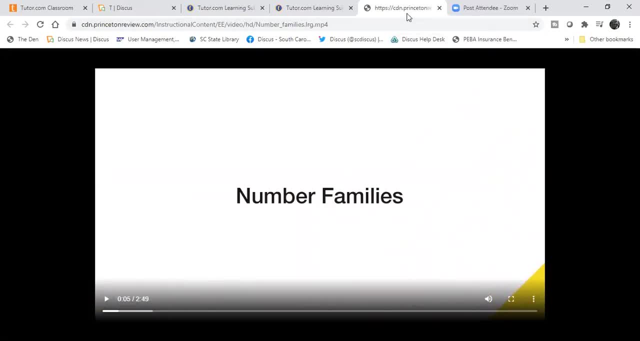 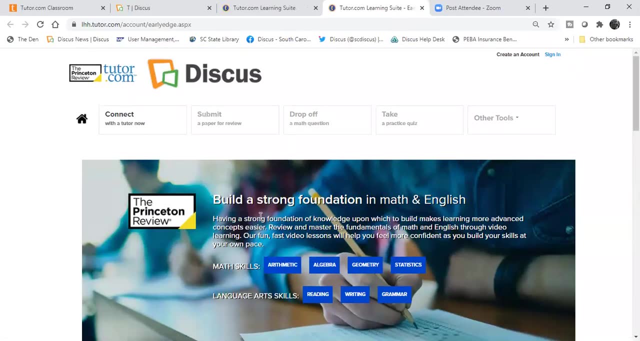 there without having to log in. So that's just another thing to keep in mind. They do have access to some of these that they can actually use And some- this might actually answer a question- where they don't even need to connect to a tutor, but just so that you know that they are there. 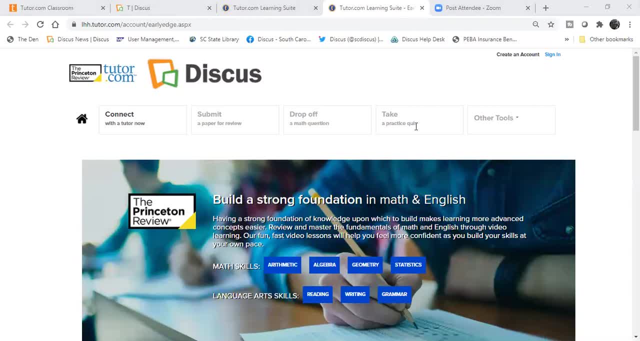 Checking chat here looks like we've got a couple of things pop up. Is a password needed to log into the SC Discus website? So if you're a tutor, you might want to check that out. So if you're a Frontline, let me go back on there. 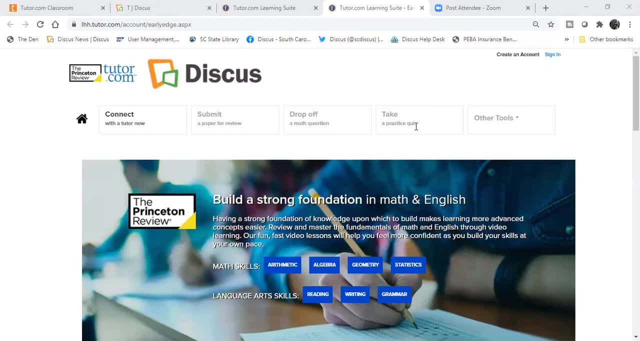 Okay, Pick a beta pass, go to the website. Can you share the ditcus username and password? So with that there is a password needed and I will be able to share that with you. when I stop the recording here at the end of the session I will share that out with Amy so that you. 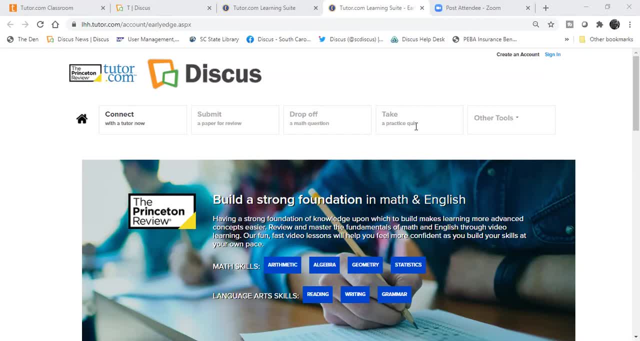 can have that, Amy, so that, so that you will have that, you can also get that from your schools media specialist and as well, if you ever need it during the school year. It changes every August 1st of every year. Thank you for your question there. 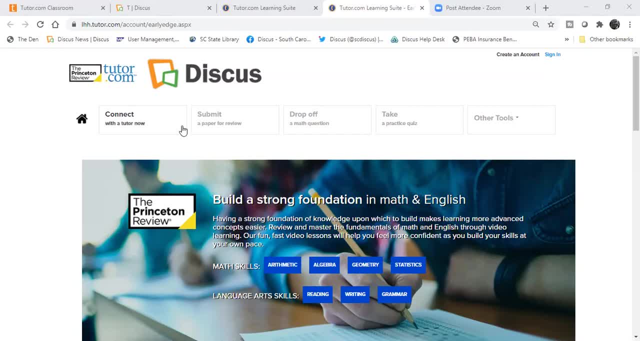 So you can see once I go. I can actually scroll down and browse what is available here, as we did with the videos. Anytime you've gone off to another piece of the website, such as that, you always want to go back to the little house that you'll see- the black house on the top. 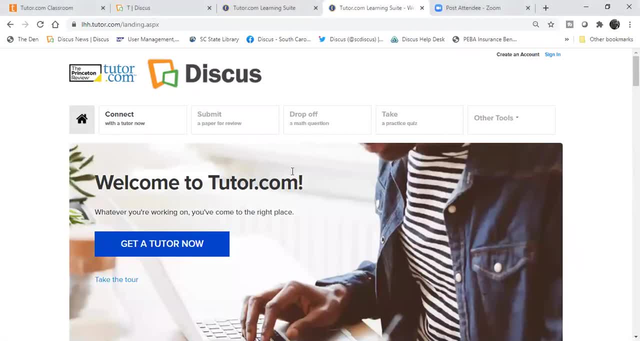 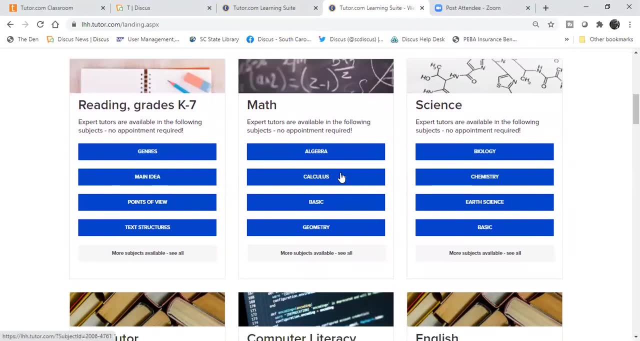 row on the left, because that will get you back to out, to that basic screen Notice down. as you scroll down, this will show you everything that's available. There are over 90 different subjects and sub-subjects- sub-categories within those subjects that are accessible. You can see this. 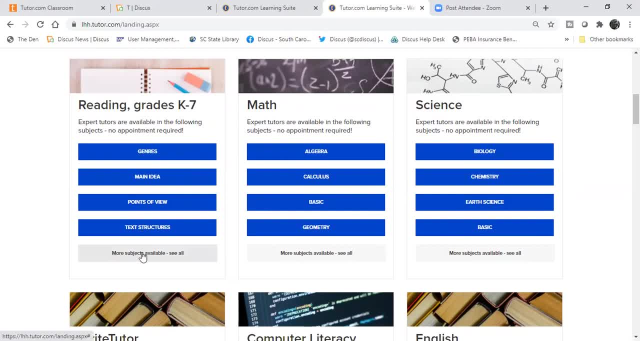 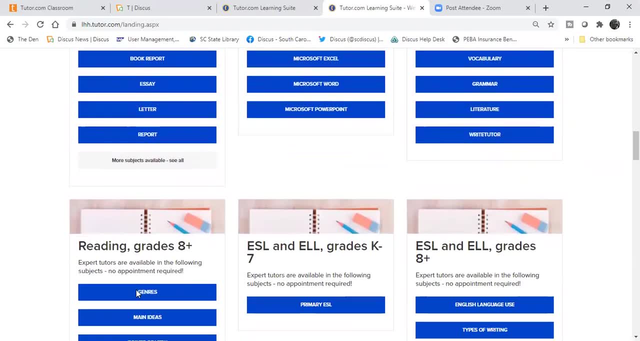 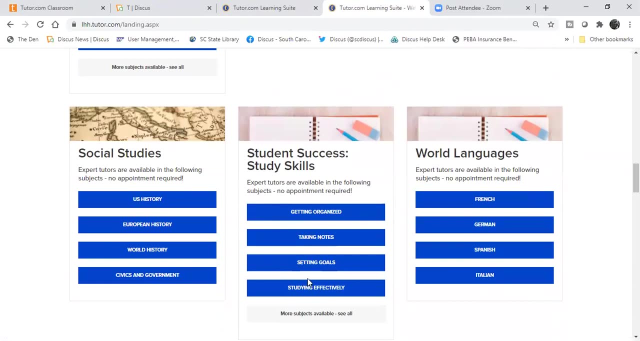 one is reading. You can go to more subjects to see what's available there. I wanted to also point out to you a couple of other features They have recently added these students access study skills. So if it's just a student that is trying to learn how to study correctly or effectively, maybe you have a fifth. 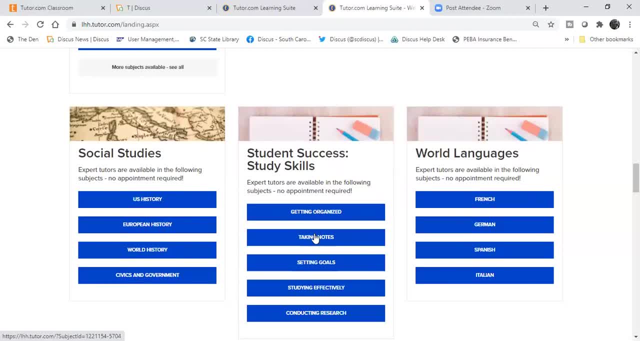 grader that's trying to learn a little bit about taking notes, etc. Those have been added recently. There's also social studies. Even though math is the primary and most used tutoring sessions that we have, there are other things that can also be of use to those students, Even a fifth grade student. 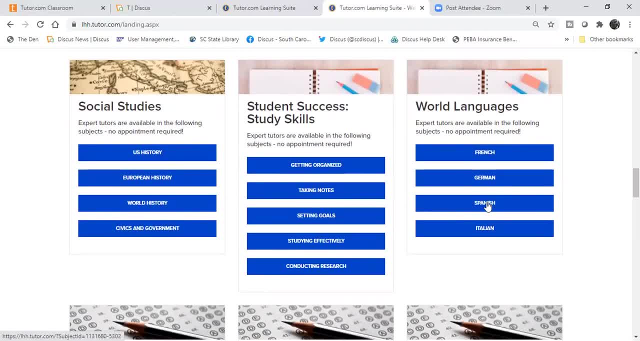 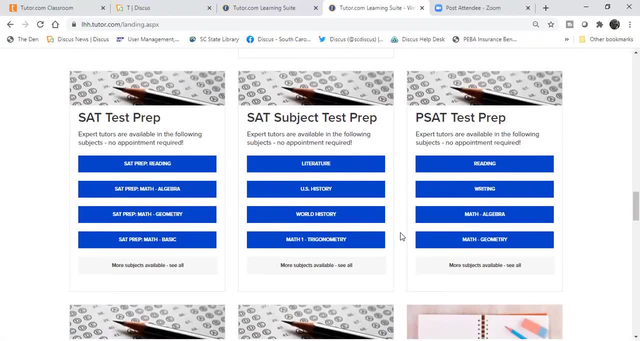 who is learning Spanish can actually log in and ask a tutor for help. You can also find a lot of these here. as you see are going to be more for your high school level student, But notice on the right here you can see that there are a number of different things that you can do here. You can: find a lot of these here, as you see are going to be more for your high school level student, But notice on the right here. you can find a lot of these here, as you see are going to be more for your high school level student, But notice on the right here. 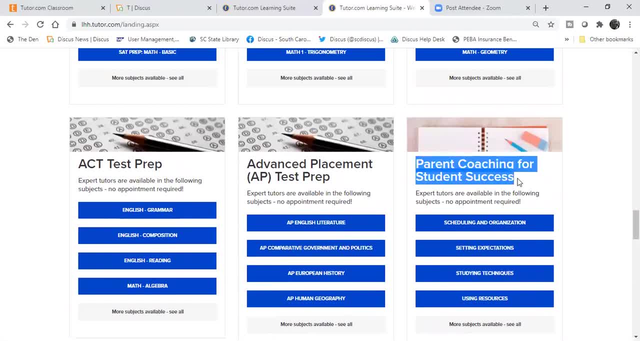 you can find a lot of these here. as you see are going to be more for your high school level student. But notice, on the right here, as I scrolled down, the parent coaching for student success. This has recently been added as well. 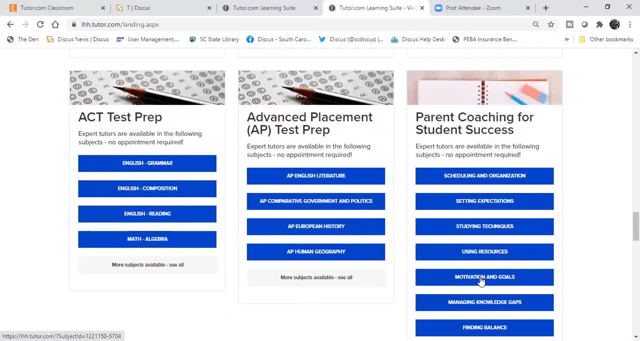 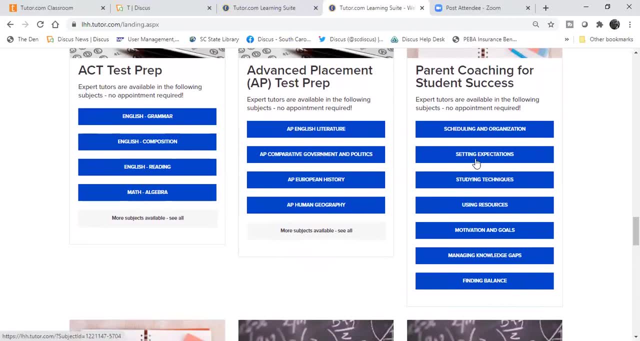 because there are so many parents, as you know, who are at home trying to assist their students- Maybe it's been a minute since they've been in school themselves- So they can help setting expectations, motivating and goals, finding balance between school. you know when to get off. 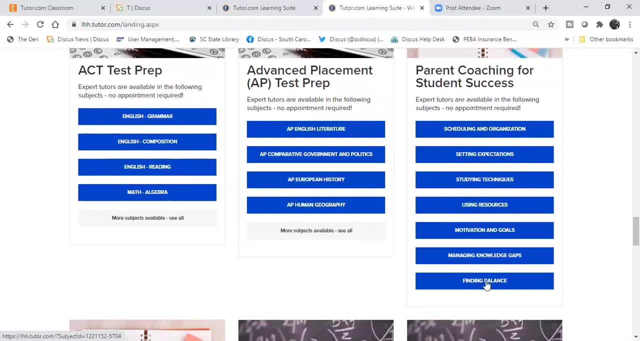 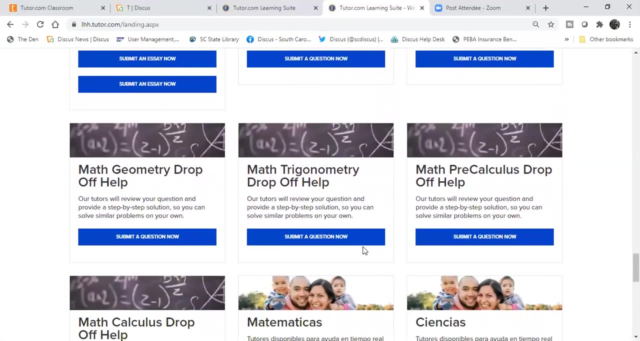 that screen time when to kind of get away and take a break. So these are going to be actually pieces that the parents can speak to tutors about to get some additional assistance with, And then the rest of these that you see at the bottom are going to primarily be for your high school level students, But we 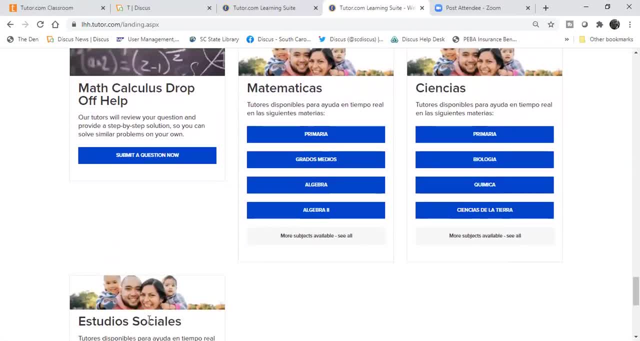 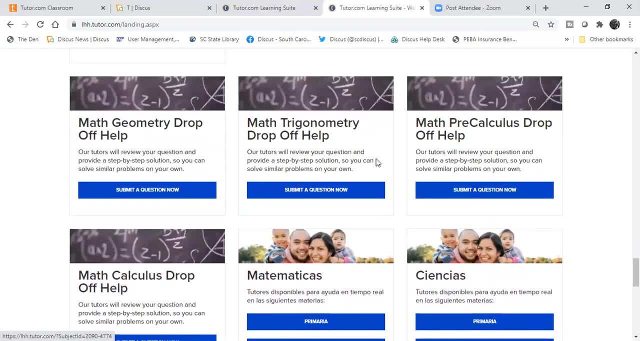 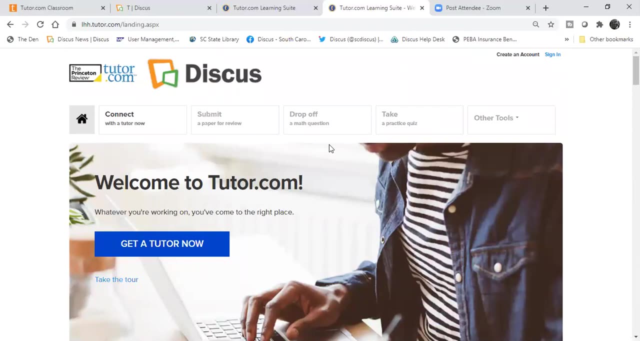 do also have the tutoring. that is in Spanish, as I mentioned before. If that is the native language of a student, they can also use these, So they can browse those categories, Or what is best for you to show your actual student is just to go to. 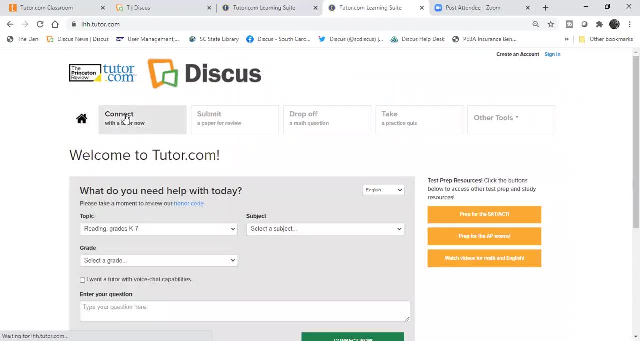 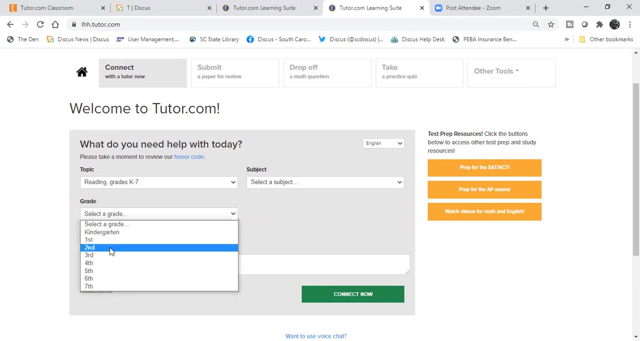 connect with a tutor. now, That's when they're going to get the ability to connect with that tutor And it's going to be easy for them to then show which grade level that they're in: kindergarten through six. there for your set, You know if they're looking at, let's say, 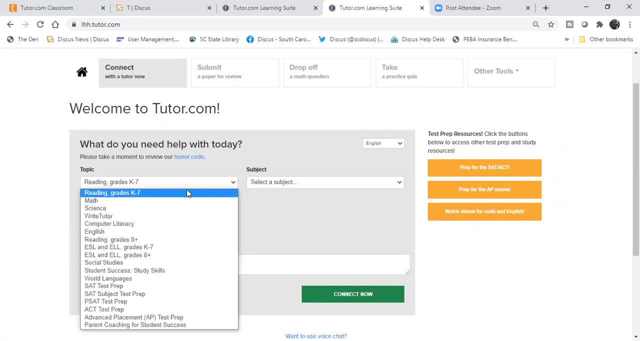 fourth grade. They can choose the topic here. They can choose their math. Once they've set those two, then the choices over here are going to change according to the grade level they're in. So if they're just wanting they have a basic math question, they can go in and enter here. 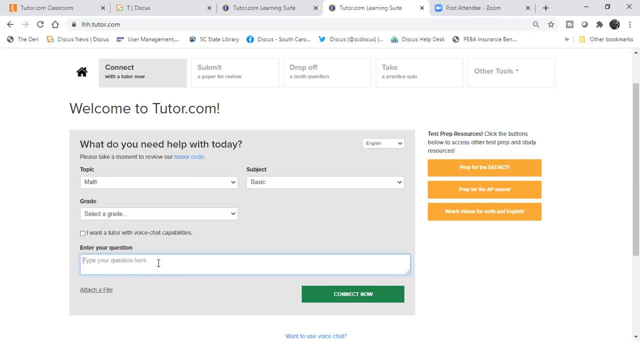 enter. you know their question. If they're having trouble with working with a word problem, they can just say: word problem, need help there to fill that in, And then they would just connect now. And we're not going to do that right now because we obviously aren't going to. 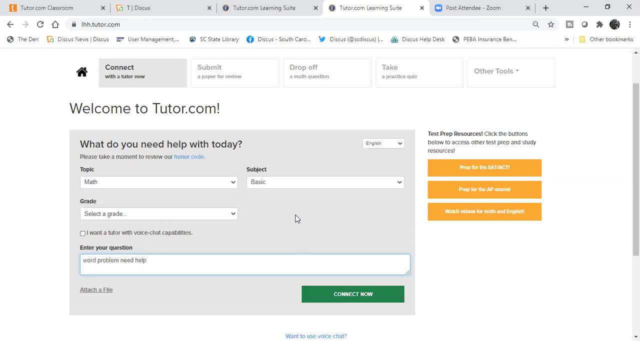 connect to a tutor to do the math, But just so that you can see how to set that up. That's how you would actually go through the process to set it up. If a student does go, you know, if they do happen to browse, then that's going to be a helpful tool for you. You're going to be able to go to the. 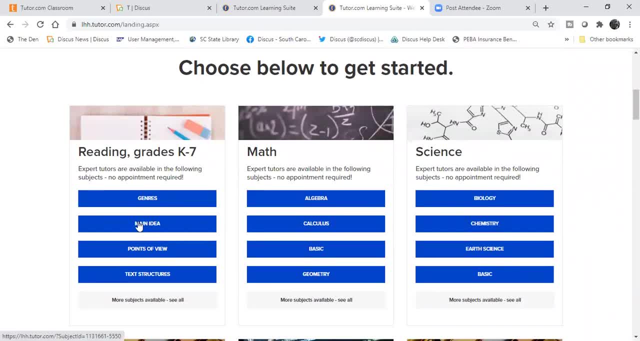 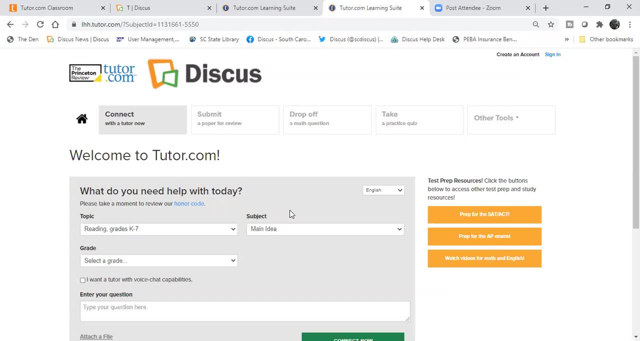 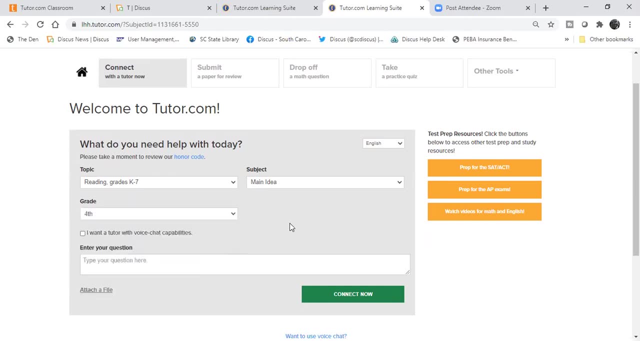 some of these little buckets down here and they want to, you know, learn about main idea in reading. when they click on that, it's going to take them to that same screen and all they'll need to do at that point that says reading main idea is tell them what grade they're in. okay, so you can see. 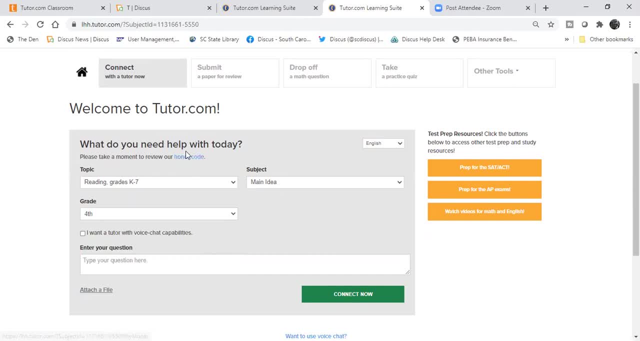 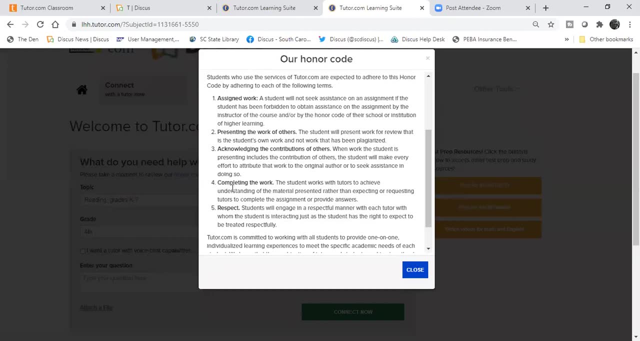 also I like to point out there is an honor code that is here just under what do you need help with today? and it does emphasize. I especially like to show you number four: completing the work. the student works with tutors to achieve understanding of the material presented, rather than expecting or requesting tutors to complete the assignment or provide answers to. 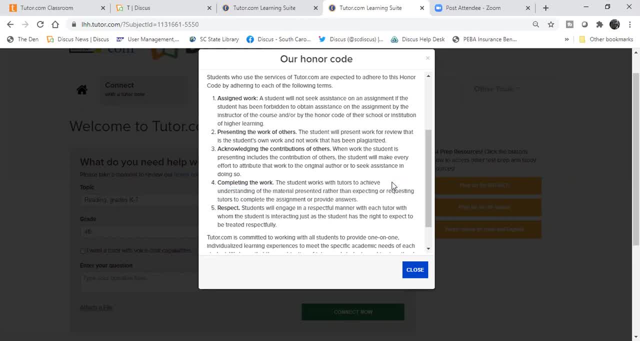 the assignments. so again, those tutors are trained to coach that student step by step, ask very specific questions to help them customize the assignment critically, think through the piece. So it really is tutoring them in order to get them to be able to understand the concepts, or understand. you know what they're doing there. 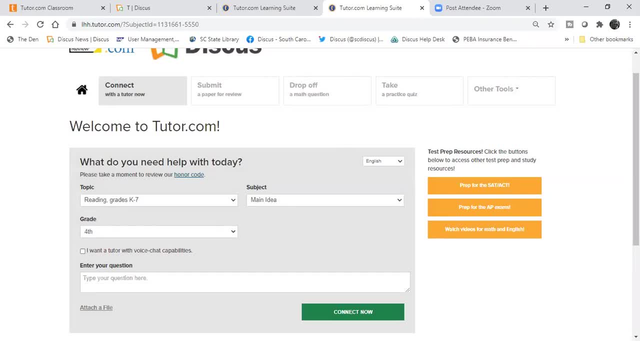 I'm going to check chat here to see if there's any other comments or questions that you have posted. Okay, not yet, So I'm going to show you one more piece here. I'm going to actually take you into the tutor classroom that your student will see once they connect with that. 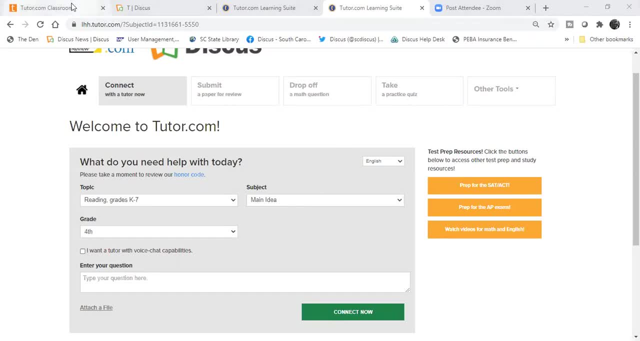 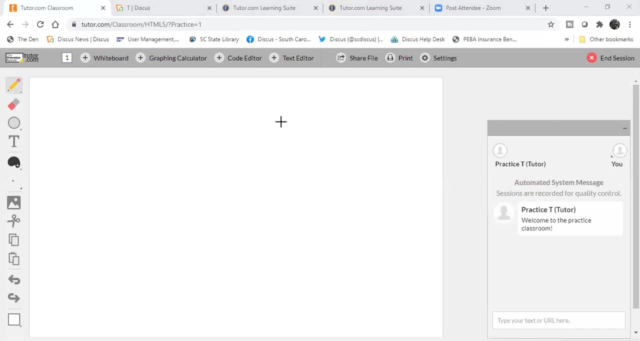 tutor And I'm just going to go ahead and change to that tab for you to be able to see this. This is just a little demo tutor classroom so that you and the parent would be able to see what is going to happen next. So at this point the tutor will have already received the information. 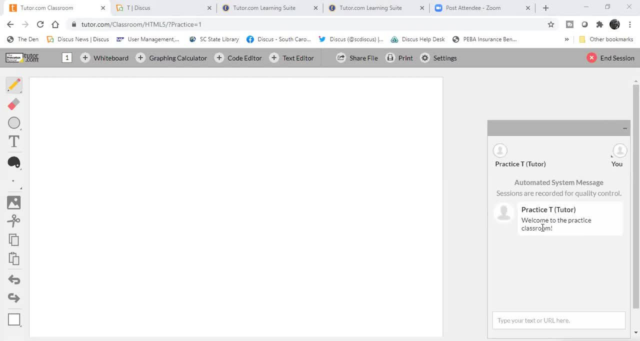 about what subject and what grade level the student is in And they will begin typing in chat here And all of this is going to be anonymous. Of course, the tutor is not going to know if you know if the student is male or female or anything about their name or any. 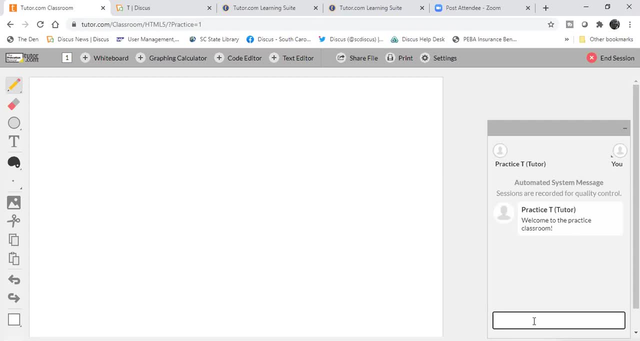 personally identifying information Because, again, they've just connected anonymously. But then the student could say: please help with this word problem here down in chat. Okay, Again, some of your younger students are going to need that parent or guardian you know, or big sister or someone in the family that will help with some of this If they aren't able. 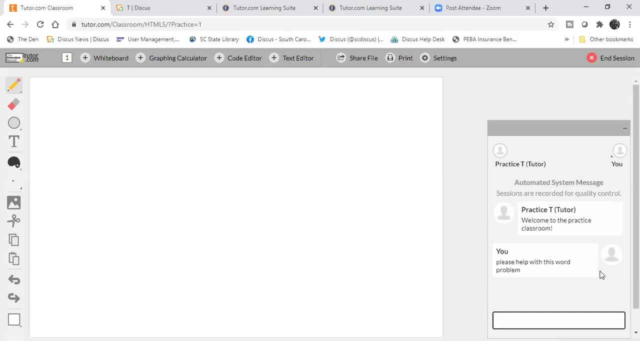 to actually type all of this out. So they will need some assistance. But again, I'm just going to say: you just kind of go ahead and write a note on of what those students are doing if they're not able to clarify what you're working with. And also a little bit of a bonus, some emphasis on: 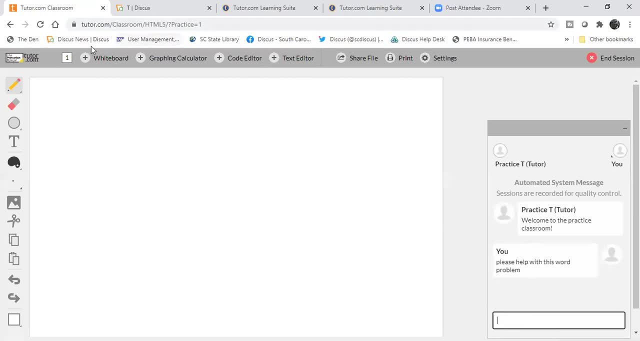 either now or then, but they will be able to find out, you know, if your student is on the elementary level, what's the course to go back to, what's the course they're doing, in advance. Then the tutor would respond back there. Also, notice: within the classroom there are whiteboards. 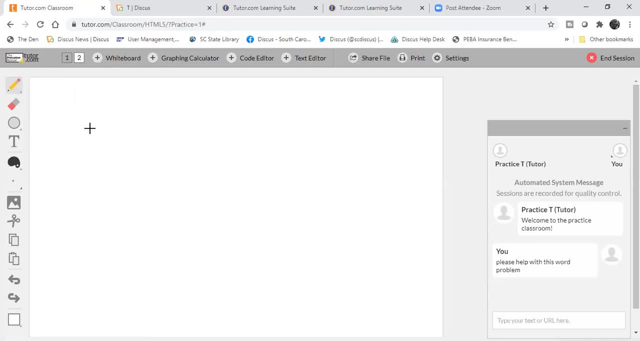 here that they can use. They can use more than one, So if they need to show a student, maybe write- know what do you have here and you know. you know what are we working with. and they can do it with with their pencil here. they can also use all of these tools on the right to be able to. 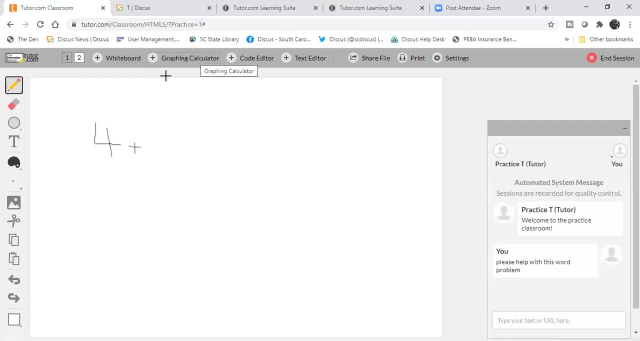 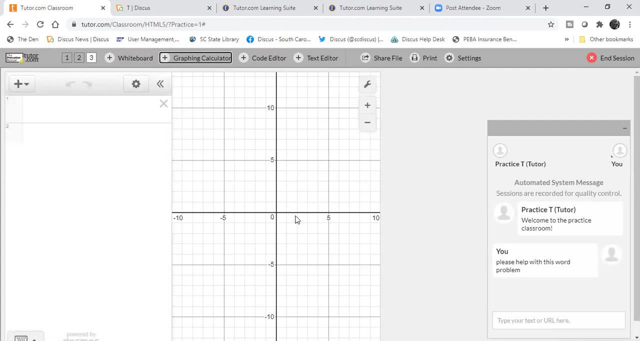 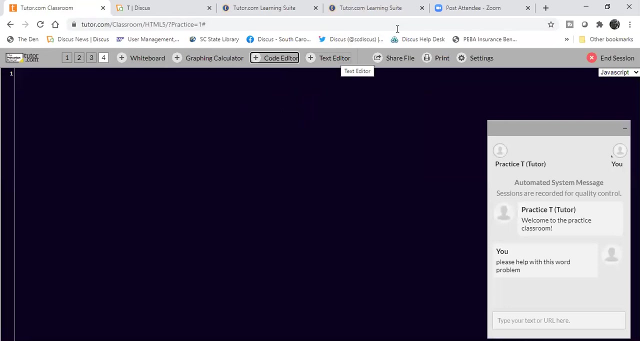 walk through steps with a student. there's a graphing calculator here also that they can use, which will be apparent here in a moment, whenever i show you another feature: the code editor is going to be more for computer kinds of pieces that they're going to demonstrate and use the text editor if the student is, you know, learning to write maybe. 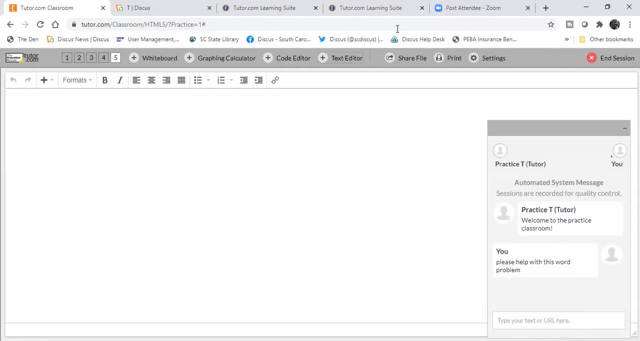 their first book report and they're struggling with a piece. with that they can actually share files back and forth, so the student may share a file or the the tutor can share a file. so there are a lot of abilities here for that. so if i wanted to share a file as a student, i could. 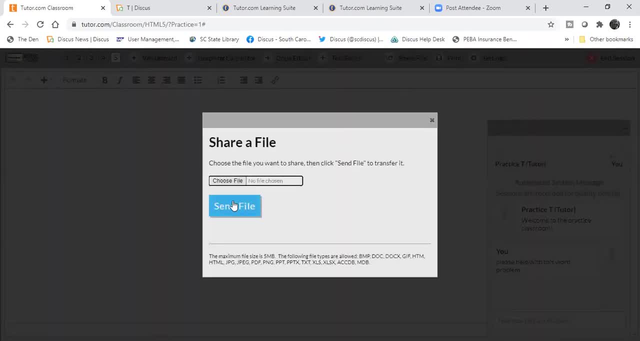 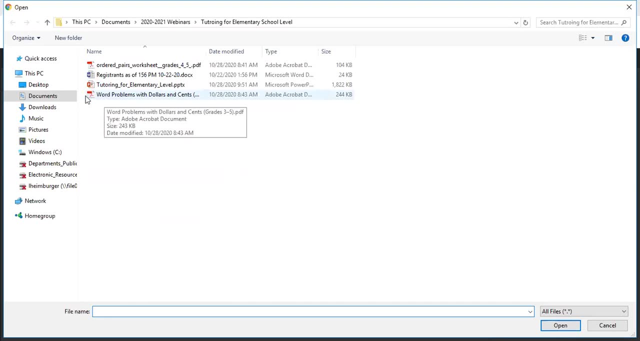 click on share file here and i could actually go out and choose that file and you might not be able to see what i'm doing now because it's a pop-up, but i will- um, i will show it to you in a moment if you don't actually see the piece, but i went out to my local computer. let's say: 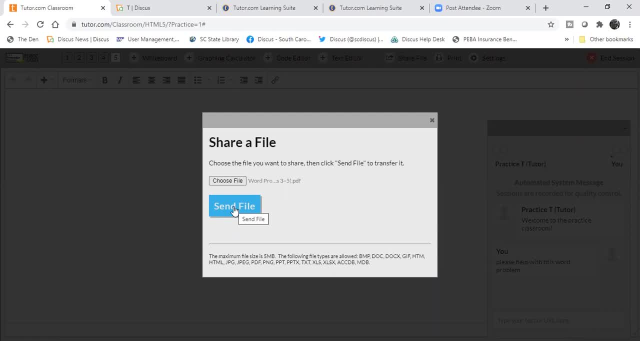 the student had an assignment that they wanted to to share with that, with that tutor. if you all in chat could show me if you see this pop-up that says please ensure the document you're about to share contains no personal information, if you could just tell me in chat if you're seeing any of that, that will be. 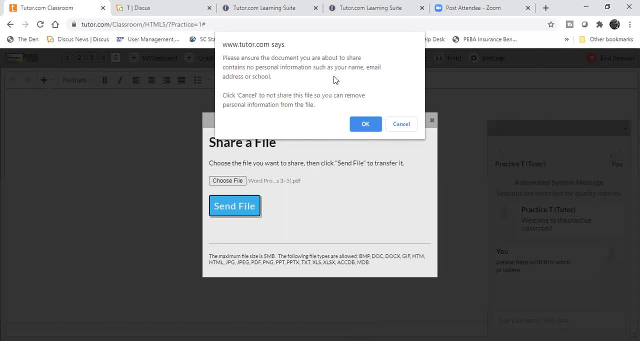 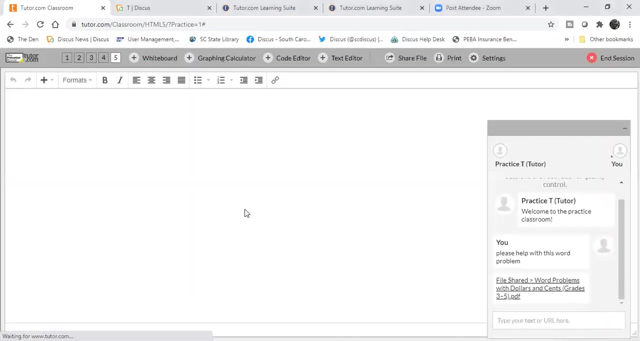 very helpful for me to know. great good, I'm glad that you can see that because that's another important piece. the parents especially- and I would, I as a parent- would also want to know that, that piece there. so once you say okay and you send that file, notice that file appears now over in the chat of the of the. 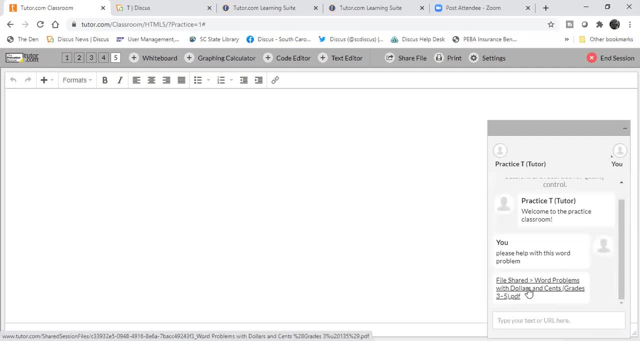 session. since this is a demo classroom, I'm not able to open that file. I'm not able to open that file. I'm not able to open that file. I'm not able to see it. but I will quickly stop share there and change it to what this file is. 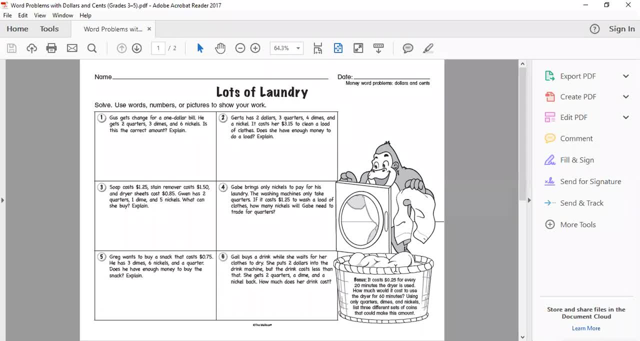 so you can see what this, this imaginary student, just sent. so this was their assignment. this is actually. this actually comes from our world almanac for kids, teacher handouts, our other database, just to show you, if they don't really know how to set up this problem to figure. 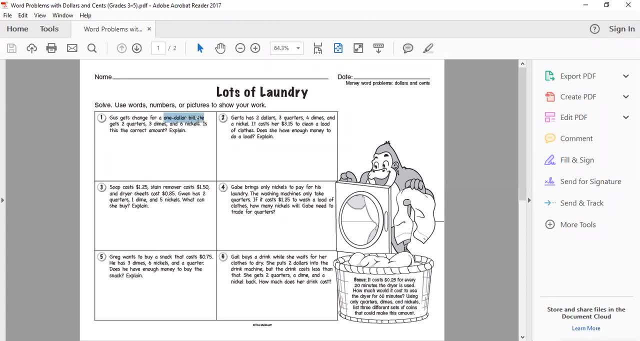 out whether or not this one dollar bill equals two quarters, three dimes and six nickels, or they don't know how to get started and perhaps the parent isn't sure about how to help show them how to do it. that's something they could do, they. 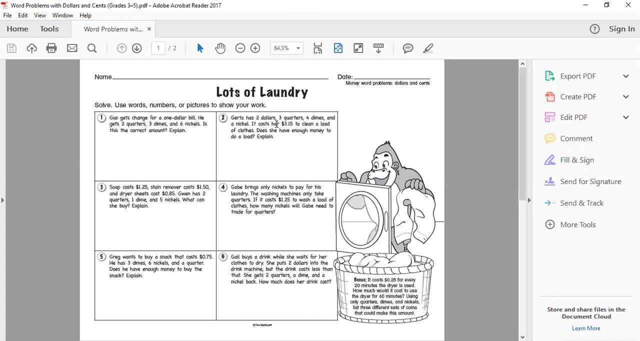 you know, they could actually share the assignment with the tutor. with that file. they could also, you know, just say: you know, I made a really bad grade on my test and I'm struggling with these fractions and I need assistance. so that's, you know, that's some of the capabilities that this does have for. 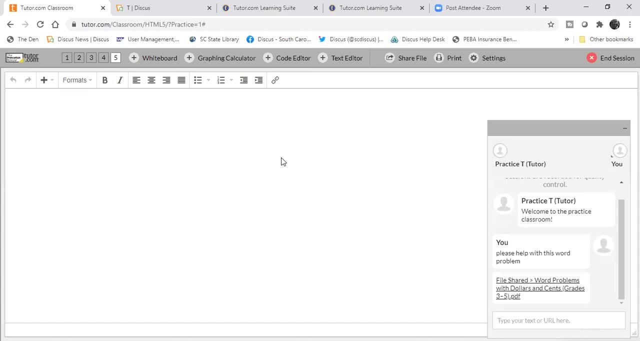 them to be able to work through pieces with. with that tutor question: if we're doing PD for our teachers, how can we show them what you're showing us right now in the classroom? excellent question, Betsy. I'm going to send a follow-up email to all of the registrants of the